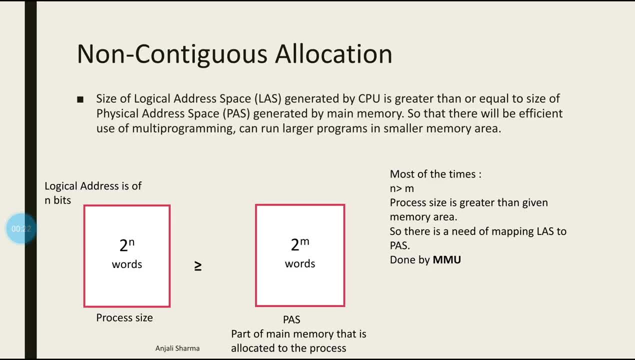 is paging Now talking about non-contiguous memory allocation. now, in order to understand it, you need to know two types of addresses, that is, the logical address and the physical address. The logical address is the address that is generated by the CPU, whereas the physical address is one which is 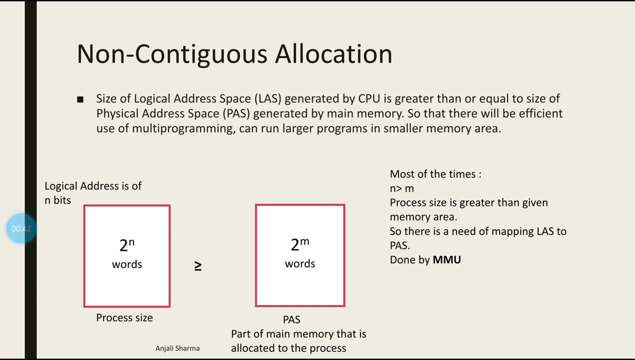 generated by the memory. So the total size of the logical address space is always greater than or equal to the physical size that is generated by the main memory. See, this can be linked with the example of memory overlays that we have started in a completely separate video. So let's start with the example of memory overlays that we have started in a. 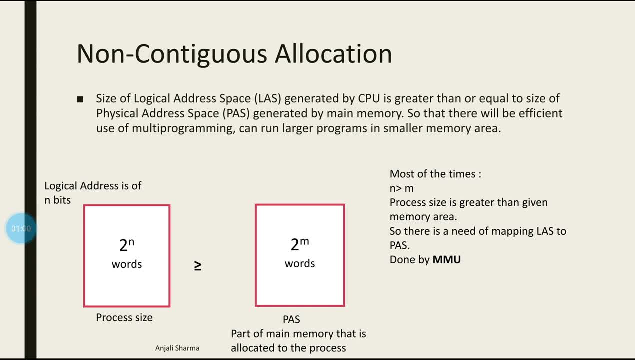 separate video and if you haven't gone through it, then go through it first, because with that you will be able to understand that. why do we need this non-contiguous memory allocation technique all together? So what actually happens, as you can see in the diagram as well- that the logical 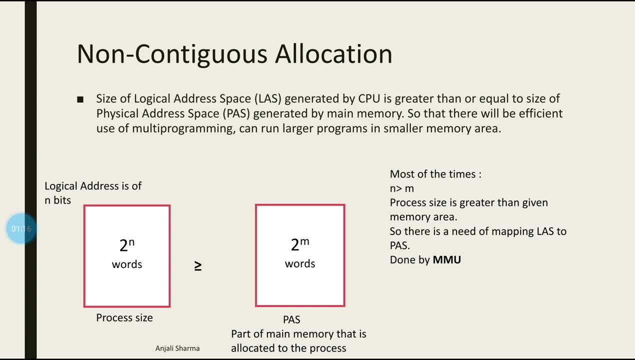 address is always greater than the physical address space, That is, the size of the program is almost, or every time is greater than the actual amount of memory that is available, So that we have seen in overlays also, For example, if I refer to that video, in that we have one program. 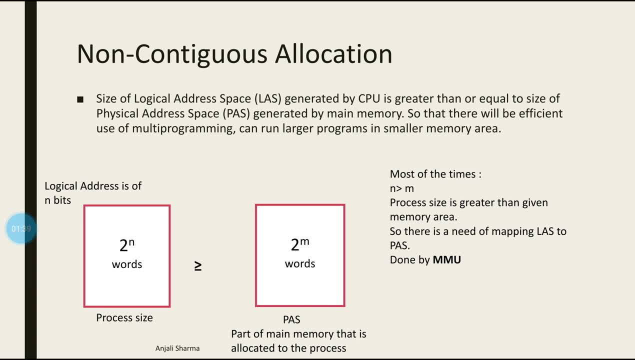 that is a two-pass assembler which is of 200k size, but the available memory was only 150, right? So we divided our program into different overlays, right, The independent sections that can be executed. So that is the basis of non-contiguous memory allocation. So it is always seen that the value of 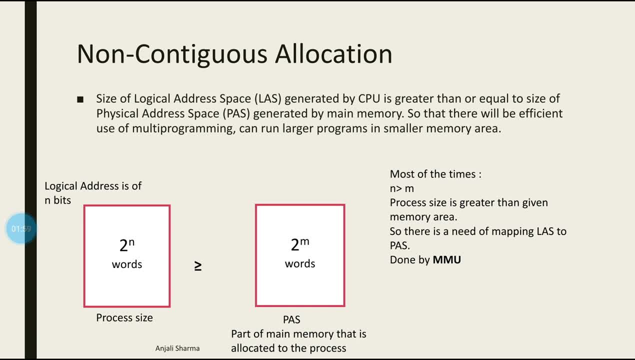 n is always greater than m, That is, the process size is greater than the given memory area. So the mapping is to be there, because we are dividing our processes into different, different portions and that will be allocated in the memory in a non-contiguous fashion. So there should be a 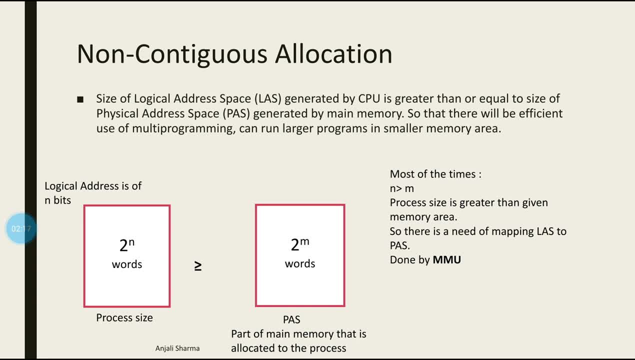 mapping between the logical address space and the physical address space and which is done by the MMU, that is, the memory management unit, And it is done because we want to efficiently to use the multi-programming technique and also we can be able to run larger programs in a. 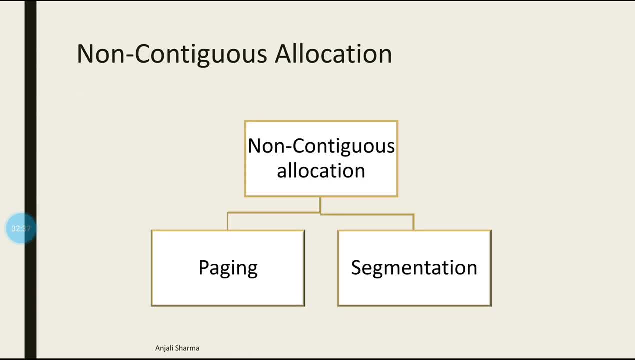 smaller available memory area. Now, talking about non-contiguous memory allocation, which is now, I think, will be clear that the program is now not stored sequentially, but it is stored in different, different chunks of the memory that can be segregated, or within the memory that can be. 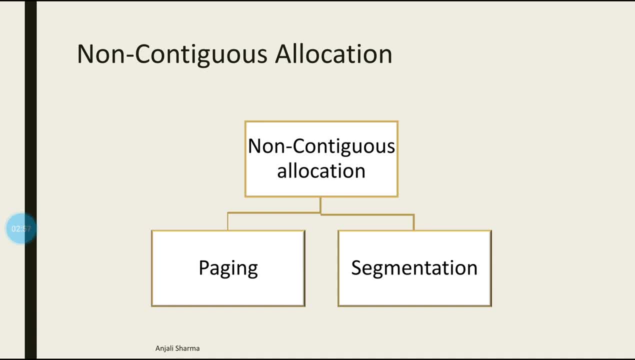 different, different portions of the memory. So non-contiguous techniques are of two types. The one is paging, another one is segmentation, which is very important as far as your university examinations are concerned, and segmentation that we will be discussing it into a separate video, and in this video we will be focusing on what paging is. 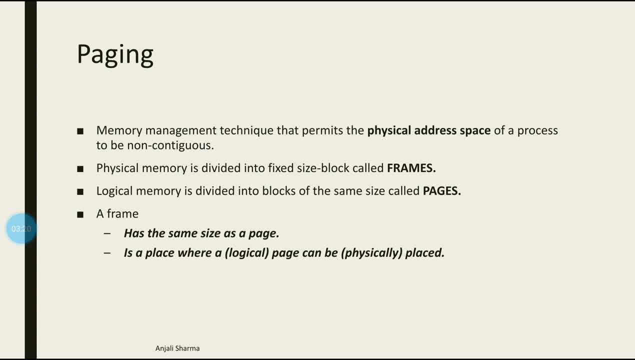 So, talking about paging, it is, of course, a memory management technique that permits the physical memory that is stored in the memory in relationship to a physical memory, in addition to the memory alignment and spiders, so that those which are stored in the memory remain intact. So what we are essentially doing is that we are actually весing the memory. 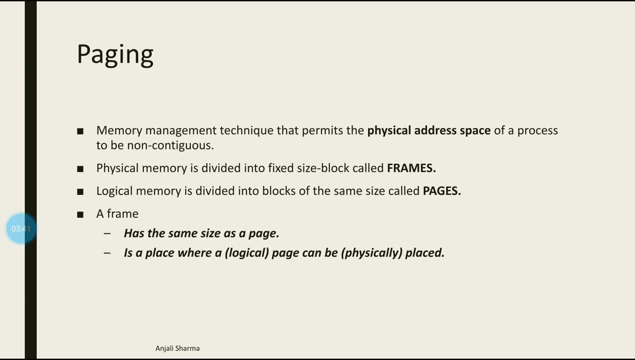 So to do that, we are using well known memory application. So there you go. Actually, I'm going to show you a little bit more detail about the method of using it. If you have any questions, please feel free to ask. If you have any questions on how to do it, please let us know. 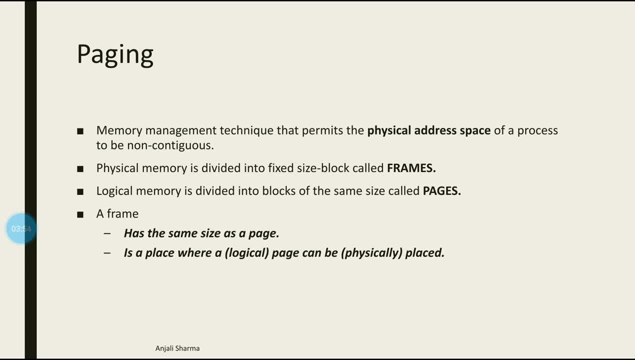 If you have any questions, please feel free to ask. We will have a question, So I want you to share this, So it's a very useful method. If you have any question or any other question you would like answered, please do so. 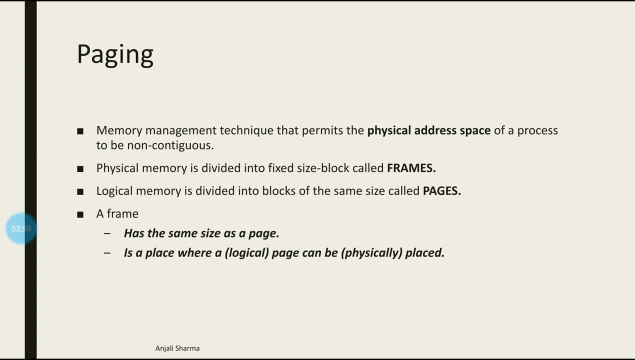 also divide the logical memory into again the fixed size block which are known as pages, and it is to be noticed that both the size of pages and frames is equal. and it is also very important question that why the page size is equals to your frame size, because it avoids internal fragmentation. 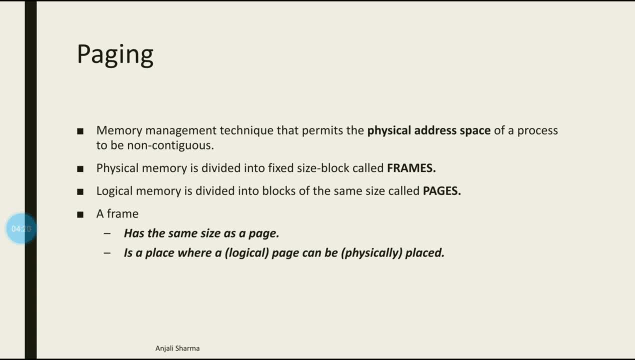 because if both the size are same, for example, again remember the previous video of internal fragmentation in that we have a chunk of 10k size and a 8k size- process came and we just applied it into that particular chunk and the 2k size memory is pasted. and similarly was an example of a 5k. 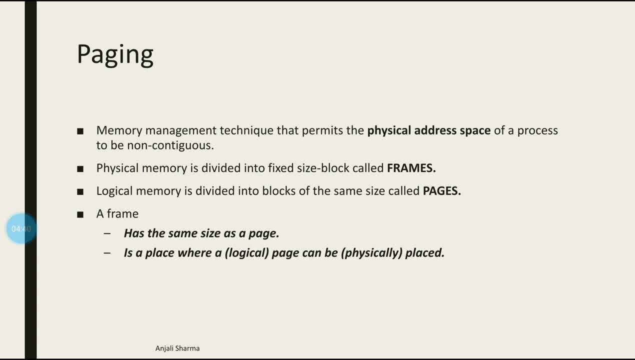 size right. so if there will be the same size of blocks in both the types of the memory, then it will be able to eradicate the drawback of internal fragmentation. but of course a paging do not completely remove internal fragmentation. the last page of your program that can be left will be obviously somewhat smaller than your frame size. 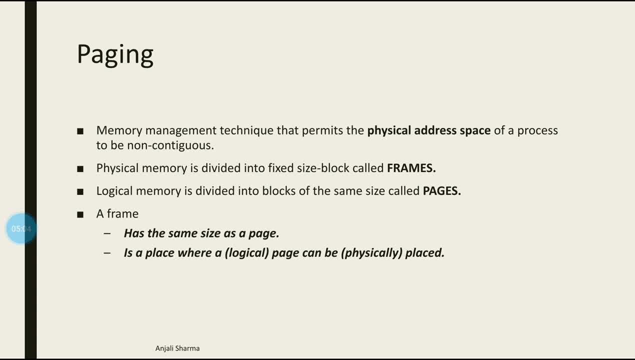 so we will be reducing internal fragmentation, rather, we will be saying that, completely eradicating another thing, that a frame is something which have same size as that of your page and it is a place where we can place our page in right now. so what exactly we are going to do in paging? 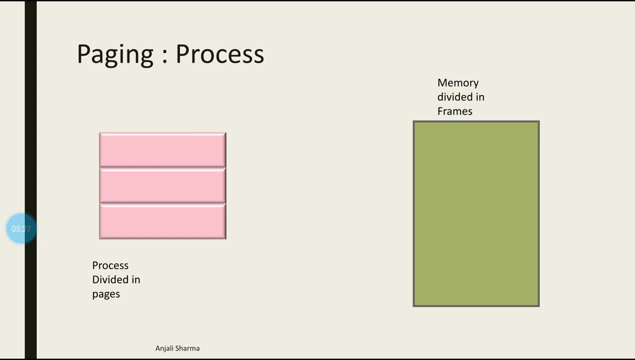 we can understand that with the help of this illustration. it says that we have a process and we have just divided into different, different pages. here we have three pages and suppose we have a main memory which is also divided into certain frames, right, of same size, right, so what? 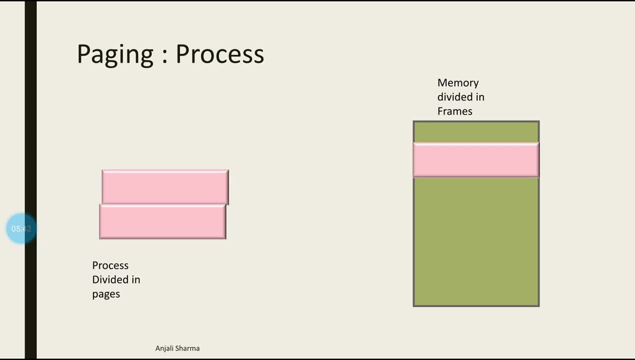 is we are going to do. we are going to place different, different pages into different, different memory locations which are available at that particular point of time. so this is the nature of non-contiguous allocation. see, the whole program is going to be divided into different, different memory locations which are available at that particular point of time. so this is the nature of non-contiguous allocation. 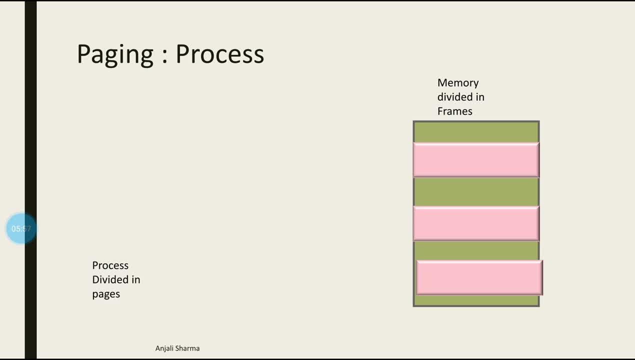 is not stored sequentially right. it is distributed among the memory right. whichever frame was free at that particular point of time, the pages will be settled into those frames. now here we are removing the concept of compact compaction, which took a lot of overhead, and also we are avoiding internal 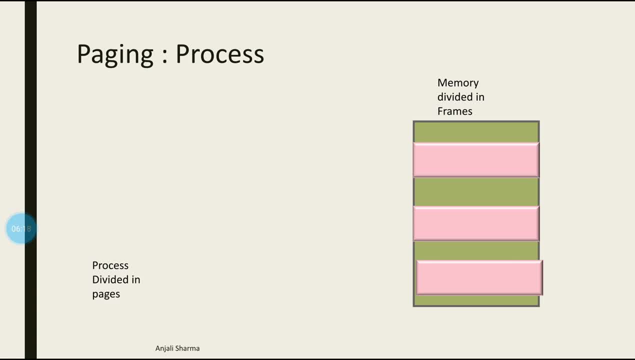 fragmentation. so paging has its own advantages, right? so this is, uh, an example of non-contiguous memory allocation, where these pages are segregated. so the first thing we are going to do is we are going to amongst the free available frames. Now this diagram which you are now seeing on your screen. 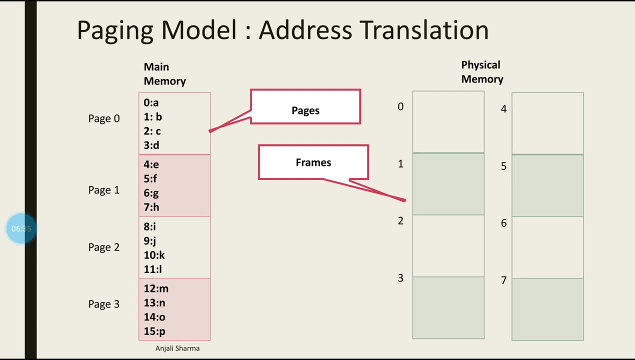 is very important and this is the method of address translation, that is, we are now going to see how the MMU, that is, the memory management unit, translate the logical address which is generated by the CPU to the physical address. and if you are a little bit confused, that what a. 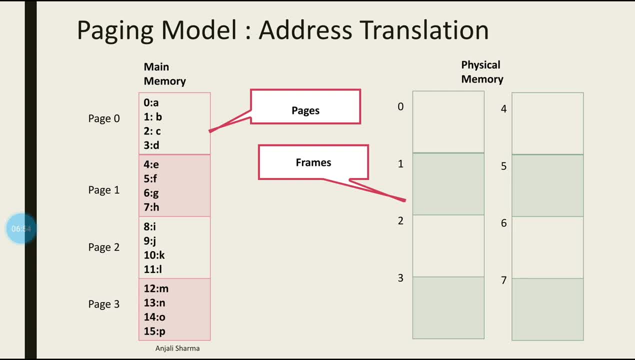 logical address is or what a physical address is. that will be cleared with this particular slide. So just have a look on the left hand side that we have a main memory and in main memory you can see that there are certain data which I have written in this. that is, 0s to 15, and there are certain 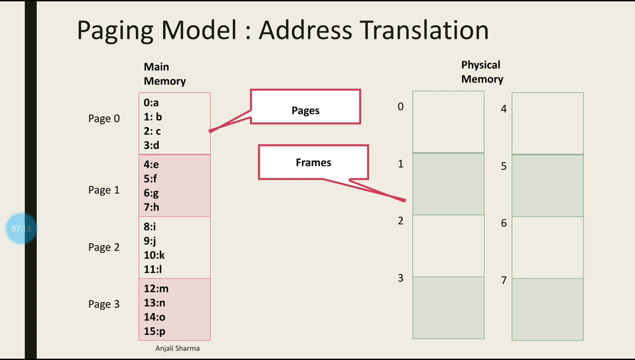 alphabets. that is written in front of them, from A to P, Right? so what it is. consider that the main memory has a physical address, which is the memory management unit. translate: the logical address has a program written in it and the program is of 16 lines, Right? so what I mean? my main memory is: 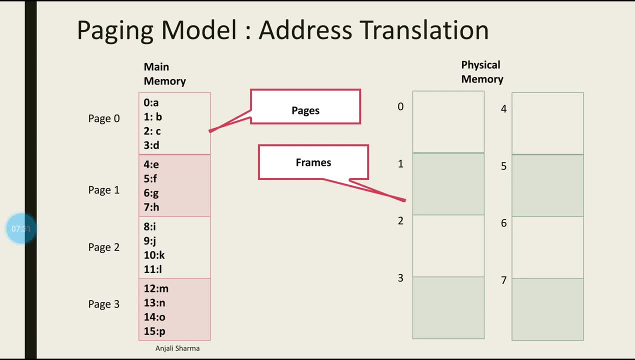 consists of? it consists of a program of 16 lines Right, and this is the indexing of line 1,, 2,, 3,, 4, 5.. Okay, and what this ABCD, alphabetic, it is the instruction of those programs. Let's say A can be. 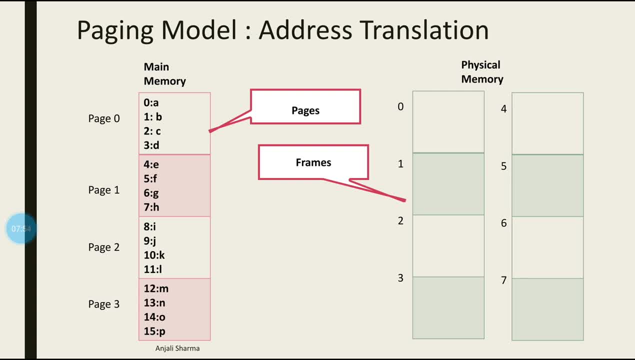 right, another header file, and C can be void main and D can be initialization of any variable, that int is equals to A and so on. Right, so consider it as a program, right instructions. So the program is of 16 lines. So what we are going to do, we are going to divide our main memory into certain 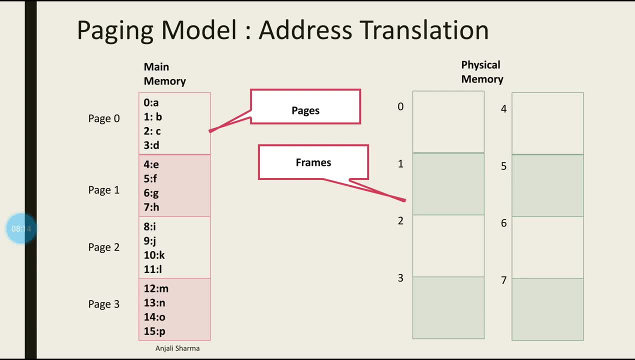 pages, Right, we are going to divide this particular program into four parts and named it as page 0, 1,, 2 and 3. Respectively, right, so main memory is divided into pages. Now what is done in the physical memory? physical memory is also divided into frame size, and the size of frame and pages equal, Right? so 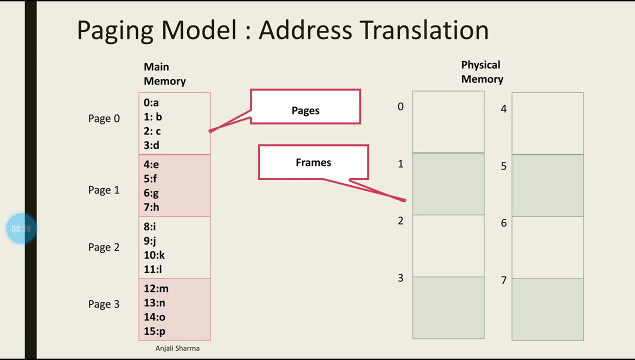 what we have. we have a physical memory and it has eight sector named from 0 to 7.. Right, so what we have to do is now we have an ability to execute our pages separately. Right? remember that page 0 is independent of page 1 and it can be put from the main memory to the 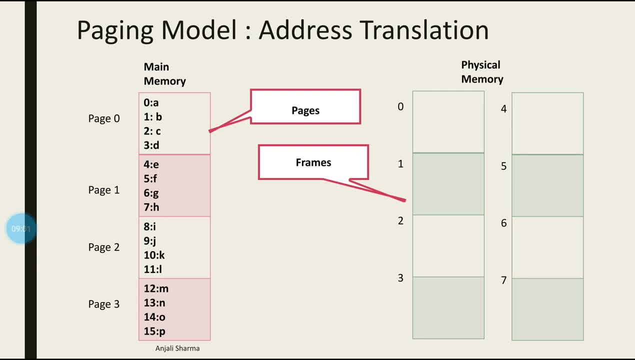 physical memory and the execution can be done as follows: Right, so what happens now? page number 0: the processor wants to execute page number 0. So it will be asking the physical memory that. is there any free frame do you have so I can put the page number 0 into that frame? 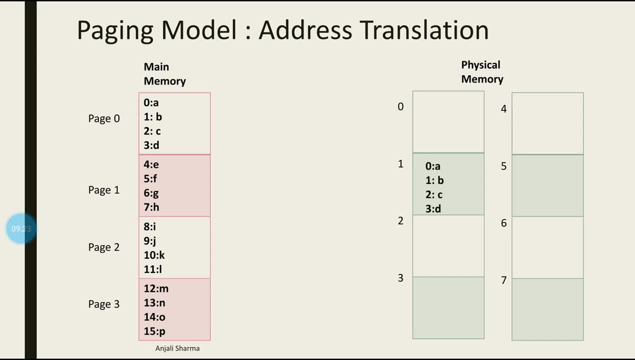 then execute it right, so it finds that page number frame number one is free, so page zero is been allocated to page number one. similarly, when the processor wants to execute page number one, it founds that physical memory has frame number three, which is empty, so it puts the page. 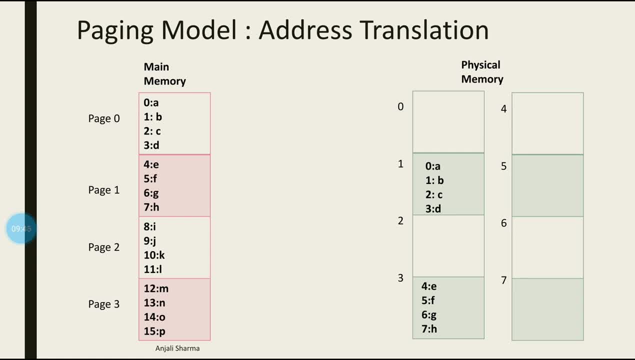 number one into frame number three. similarly, when the processor wants to execute page number two, it finds that frame four is empty and it plays it in that frame again. for page number three, it find that seventh frame is free, so it put that page number into frame number seven. so what we? 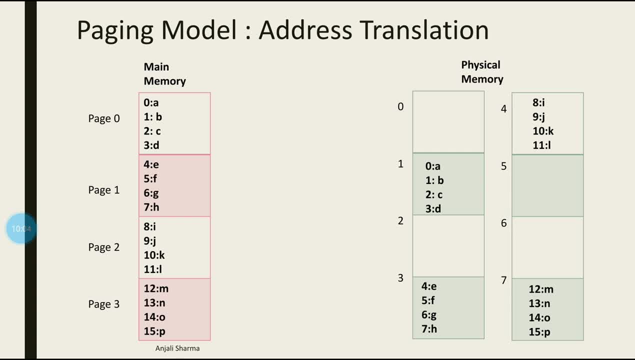 have done that. we have now distributed our pages- pages is the program- into different, different locations or different, different frames of our physical memory. now remember: the cpu generates the logical address. that means cpu knows the location of pages right and the instructions which is written in the pages, but cpu doesn't know where the pages are now being placed in the 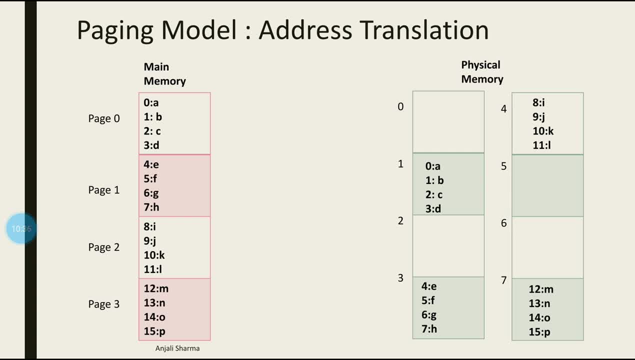 physical memory, because as soon as we get free blocks we keep our pages there. so now cpu doesn't know that where these frames are actually which are holding the pages right. so for that we have a data structure or we have a table sort of structure, which is known as the page table. 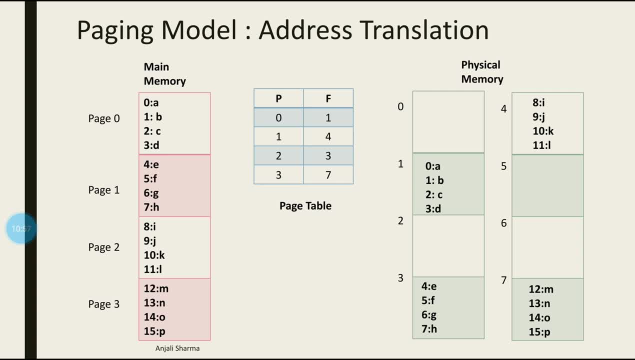 which contains the corresponding mapping of the pages with the frames right. so you can see that it has two columns: one is for the page number and other is for the frame numbers. right, we have four pages, zero to three. so page number has the entry from zero one to three and the frame numbers have the corresponding entry. for example, page number zero. 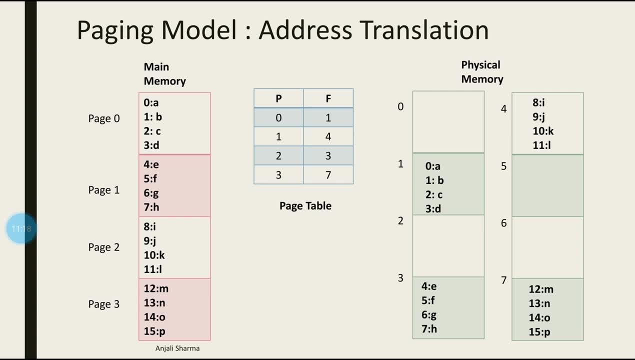 is in frame number one, so zero is corresponding to one. similarly, page number three is in seventh frame, so it has that particular entry in it. remember that the page table also have certain other entries. also that means it can have more than two columns, but there can be different, different columns as well. 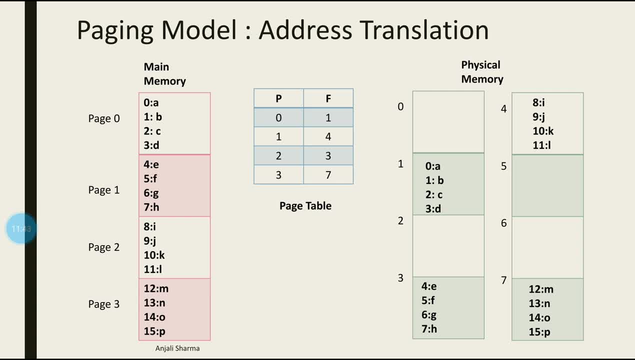 which are different. so what we are just understanding over here is that we know that where my page is residing in the main memory, but i don't know where my page resides in the physical memory, right? so here the work of address translation comes into being. so what it is done and how it is done, that let us. 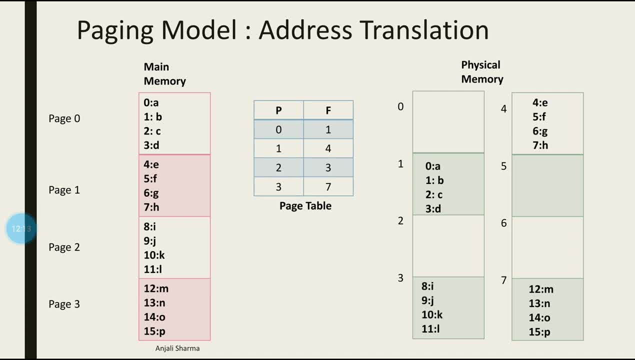 understand. so we have this particular scenario. just pay a little attention on the particular thing which we are now i am going to explain. see, what i have done is i have written the corresponding binary numbers, that is, illustrating the page numbers and the instructions written in those pages. see, i have 16 instruction with me in my program, right? so in my program i will be writing 16 instructions with me in my program. so E15C2 and Eily at 12 and Q間 14 have 23 Inspections and Quie mentioned in the primary model. so I can use these. 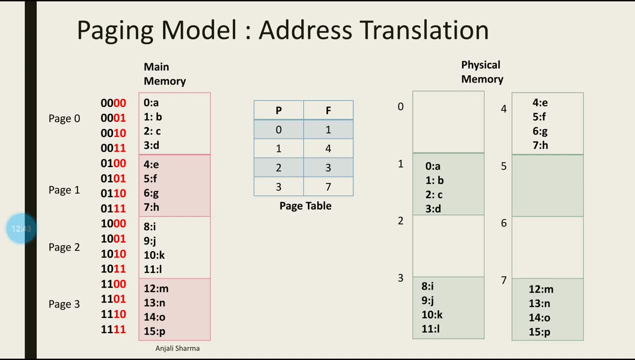 In order to represent 16 decimal numbers into binary, I will be requiring 4 bits, right. So what I have done? I have just represented the binary number of the corresponding indices. you can say, and just pay an attention, that I have used a different color screen scheme. 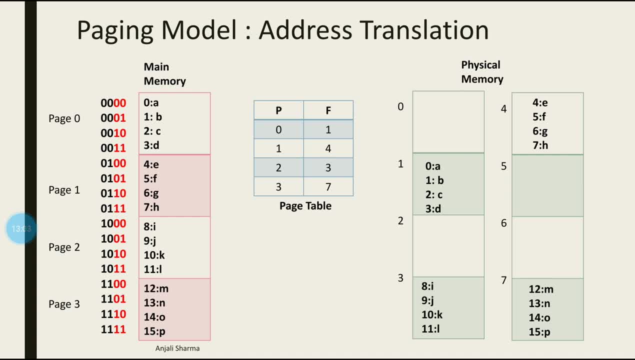 in order to represent it right, Just pay attention on the black portion of the binary number, See page number 0, and just look at the black portion right. It has 0, 0, 0, 0 and 0, 0 for both the 4 instructions from 0 to 3, right. 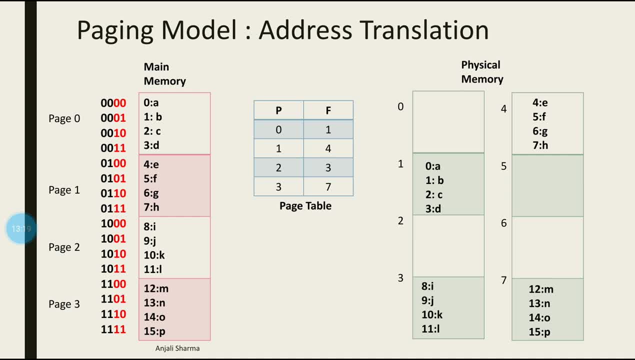 So it is corresponding to page number 0.. Similarly for page number 1 you can see the black portion. that is the first 2 bit of the binary number right. It has 1: 0. that is the binary of page 1. that is 1 is represented in binary in 1: 0 right. 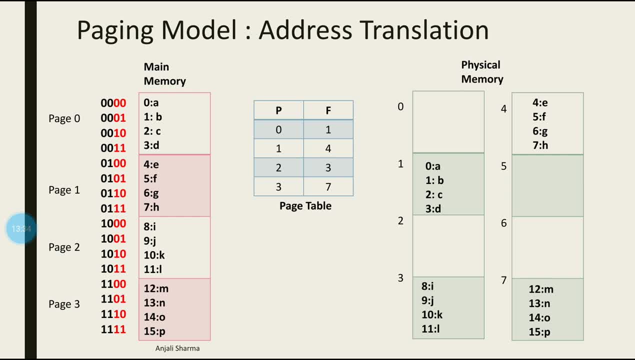 Then we have page number 2. just look at the first 2 bit, that is 1: 0, which is the binary of 2, and 1: 1, which is the binary of 3.. So this black binary, that is the first 2 digits of the binary, is representing the page number. 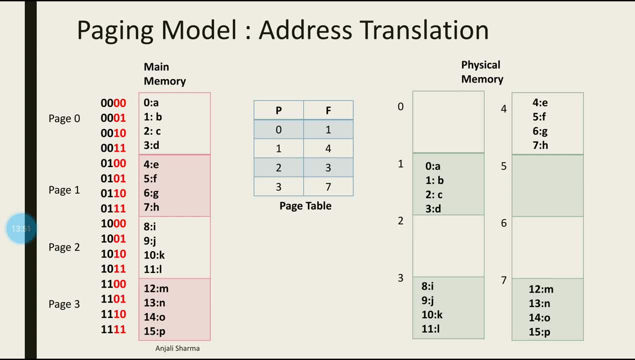 right. Now come to the red portion. See the 4 binaries are repeating 0 0- 1 0. sorry, 0 0 0, 1 1 0 and 1: 1 right. So what it is corresponding? It is corresponding to the instruction within the page. 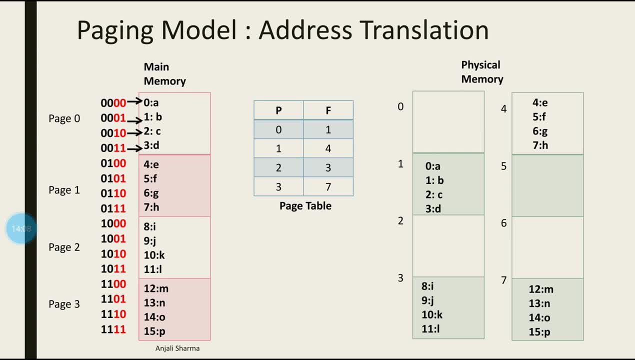 So what is corresponding? It is corresponding to the instruction within the page right. So if I have a number that is 0, 0, 0, 0, if I have 4 consecutive 0 with my, I can identify that I am talking about page number 0 and the first instruction of the page number 0. 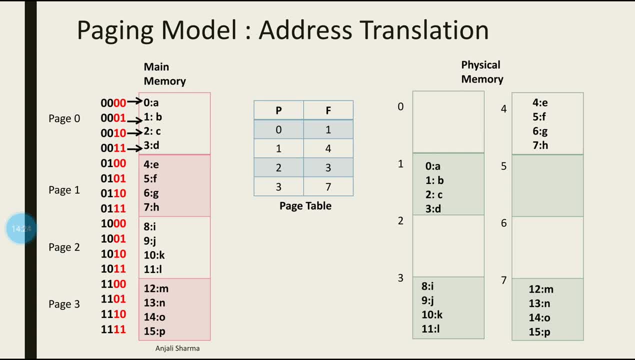 right. Suppose if I have a binary number that is triple 0- 1.. So I can understand that I am talking about page number 0 and the 1th instruction of page number 0.. So this is nothing but the logical address that is generated by your CPU, which is a combination. 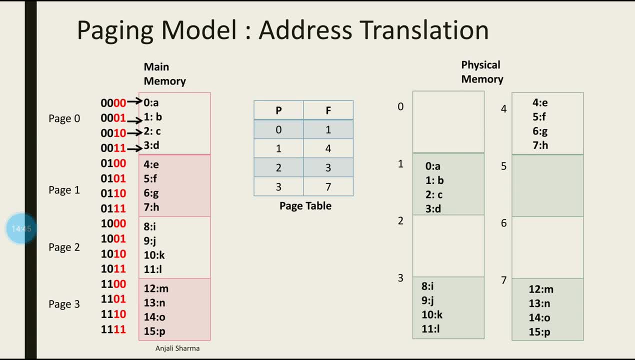 of page number and the offset: The number which is written in black color, that is the page number, and the number which is written in the red ink: that is your offset. So it basically identify the address of an instruction which is written in the main memory. 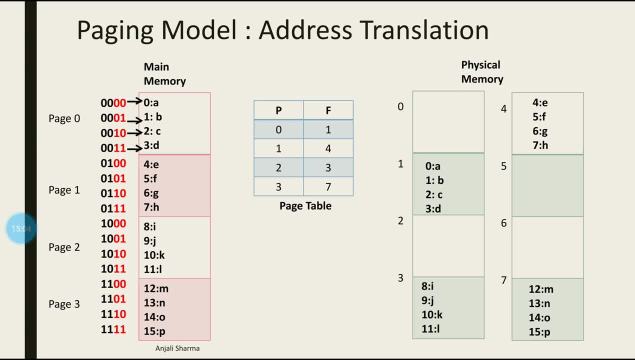 right, So the CPU has this particular data with itself, right? So what is to be done? suppose now, what CPU has to do is to execute the instruction number 8, right, which is marked by this arrow: right. So what CPU has? CPU has this address, that is, this corresponding address, that is 1 0 0, 0, right. 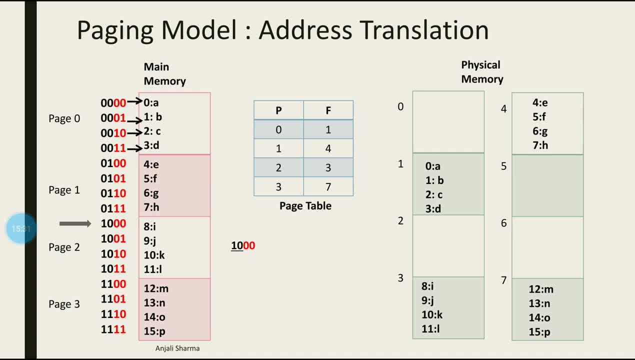 The underlined section says that it belongs to page number 2.. And underlined section says that it belongs to page number 2.. And it is the first instruction, that is the 0th instruction of page number 2.. So what CPU can do? 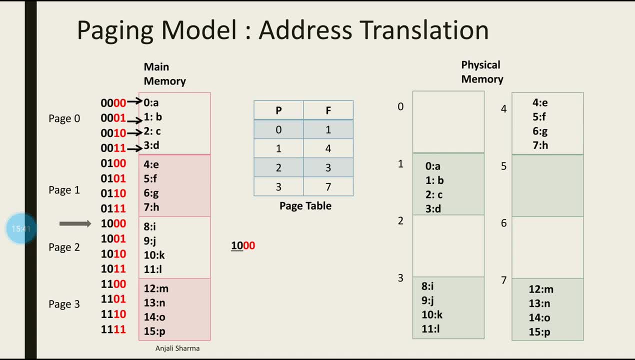 It can locate its location here, right. But now the thing is that what we have done, we have put this page number 2 into the main memory Where there was a free slot of the frame. we have kept it there. So I do not know the address of page number 2 in the physical memory. 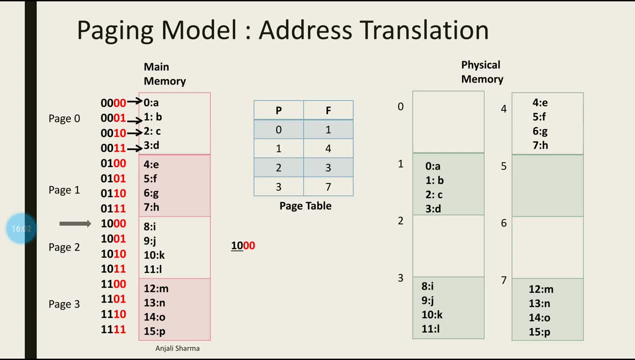 So what is to be done is that now We will be referring the page table- See via page table. I know that this underlined portion says about page number 2.. It is the binary 1: 0 and it corresponds to decimal number 2.. 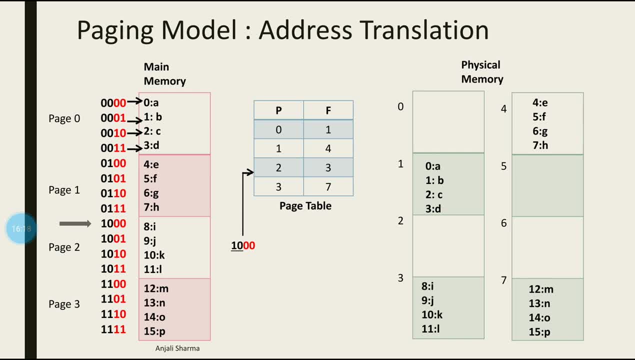 So I am talking about page number 2.. So I just went to the page table and just checked the entry of page number 2. And with that entry I can find out the corresponding frame number right. So I get that the frame number is 3.. 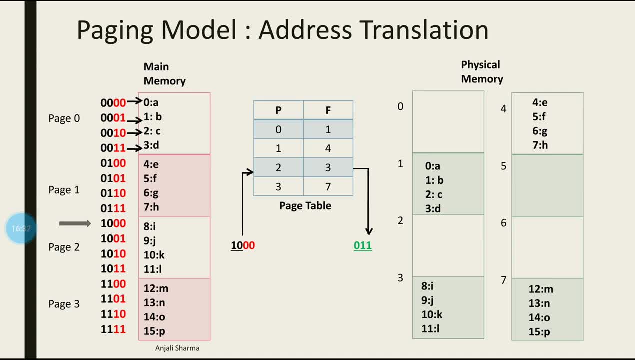 That is nothing but 011.. Which is the binary of 3, right? So now I know that I am talking about frame number 3.. That is, it is evident that page number 2 is in frame number 3.. But now I do not know that which instruction I am talking about. 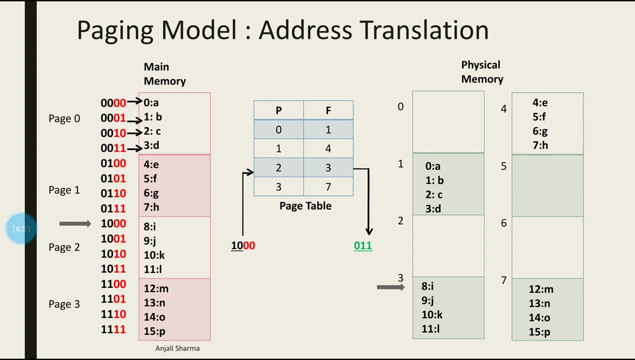 I am talking about 8, right? I do not know whether the 8 is the first instruction, the second instruction or the 4th instruction within the frame 3, right? So for that, what we will be doing, We will be combining this offset together. 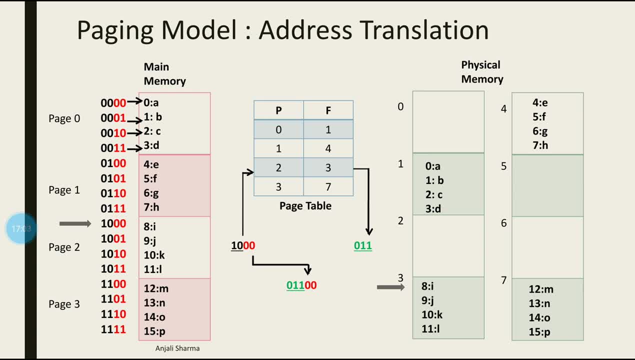 With the 4th instruction, With the frame number, right? We know that internally the addressing is done by the offset, right? So what we have done? we have just combined the frame number with the offset and now I know that 8i is the first instruction written in frame number 3.. 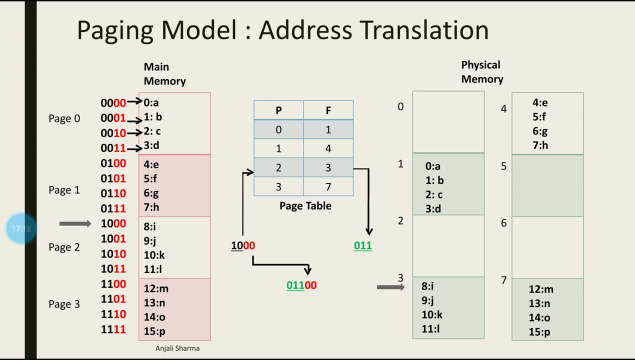 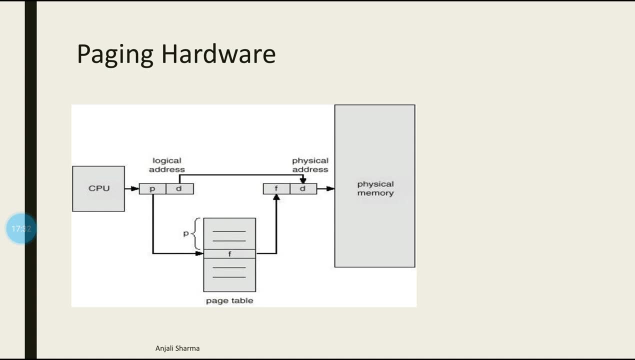 So that is the address translation. that is done in paging in order to map the logical address space with the physical address space. I hope the explanation is clear to you all now. So that is done Now in order to understand it. Let us again just revise the whole procedure with the standard diagram. 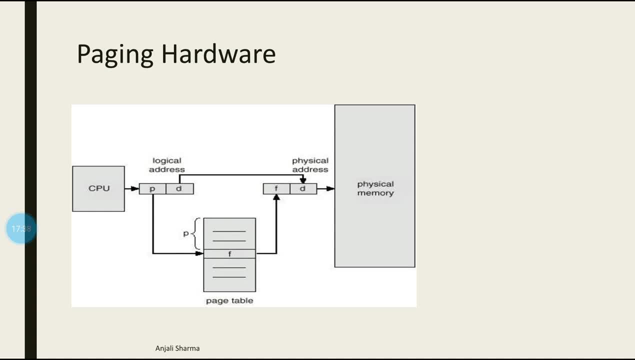 It says that the CPU generates the logical address and which is nothing but the combination of the page number and the offset. The p is the black portion, the two bits and d is the red colored bit. right, So what we are doing? we are just referring the page number in the frame table and we 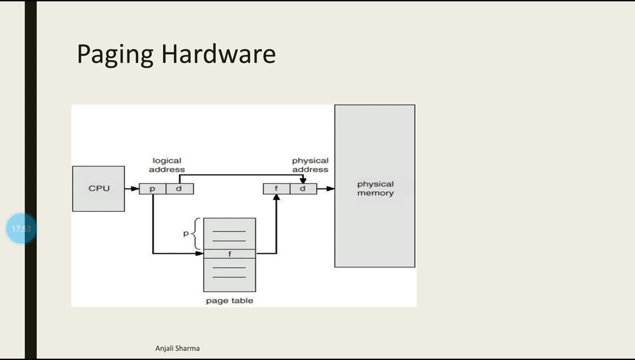 will be getting the value of corresponding frame, that is, f, and then that frame number is combined with the offset and we are again getting the address of your physical memory. So what we conclude is that the frame number is the offset and the offset is the offset. 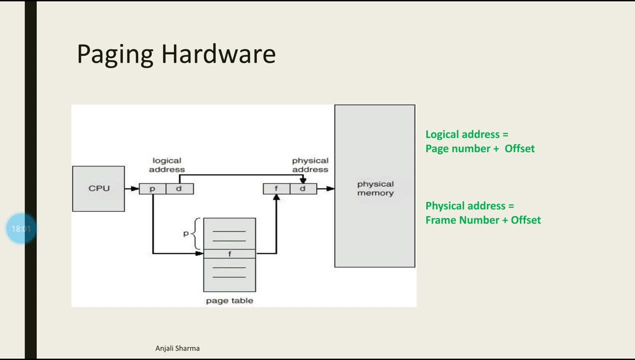 and we are again getting the address of your physical memory. So what we concluded Or what we get from this address translation? that we have two addresses: logical address, which is just the summation of page number and offset, and the physical address, which is the summation of your frame number and the offset. 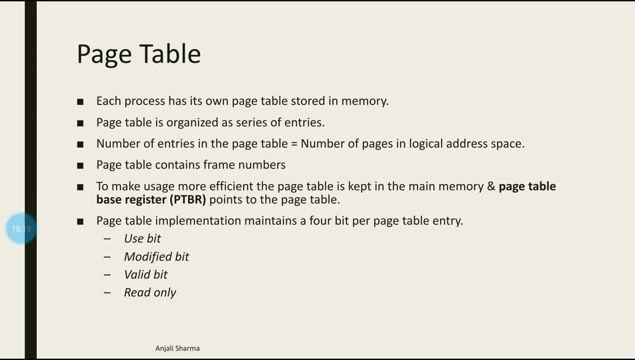 Now let us just revise or just understand some important topics regarding the page table, that is, the. each process has its own page table that is stored in the memory. The page table is organized as a series of entries. The number of entries in the page table is equals to number of pages in the logical 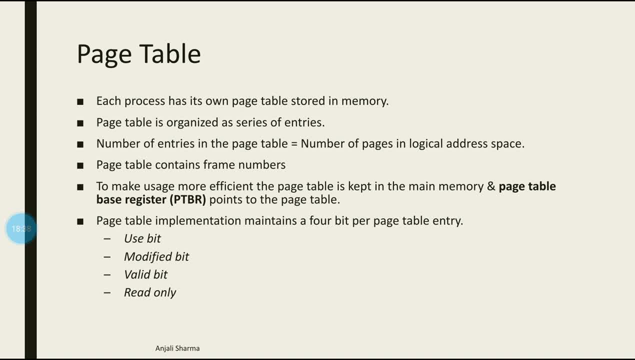 address space. The page table contains the frame number that we have already seen and, to make the usage more efficient, the page table is kept in the main memory and there is a page table base register that is ptbr that points to the page table. so each and every process has its own. 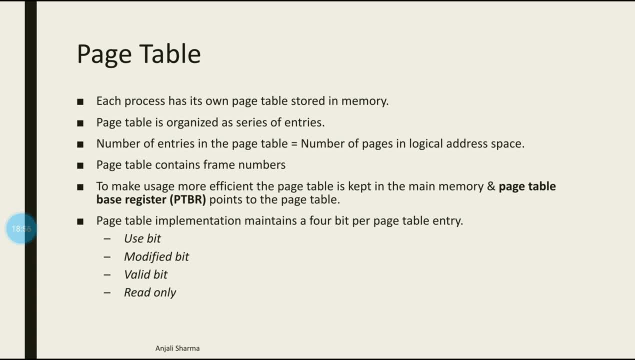 page table and in order to locate the location, we have a ptbr, that is, a register that stored the first address of your page table and that is the point that I have already discussed with you. that page table, along with the frame number, can have different, different columns. 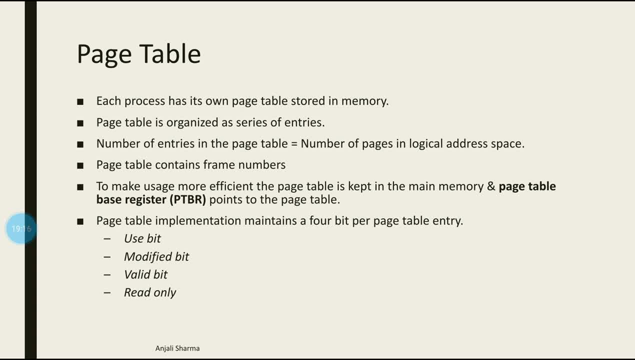 as well. for example, it can have a use bit that can define whether this page has been used or not, a modified bit that whether this page has been modified again or not, then it is a valid bit that, whether it is a valid page entry or not, or read only. we can also. 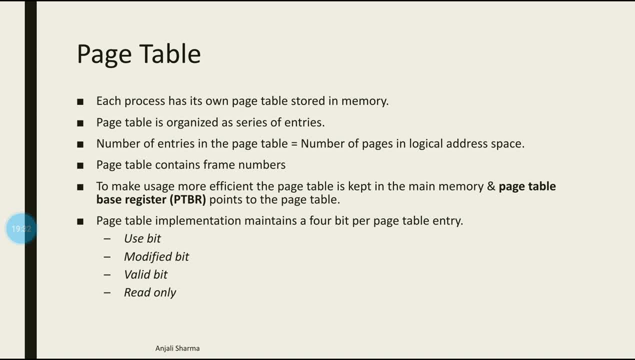 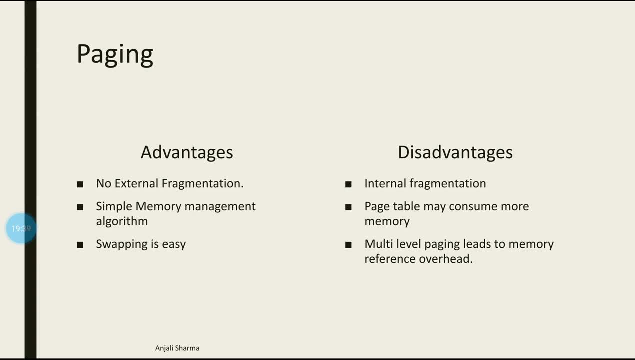 define our pages. We can also define our pages to be read only, and that is for the page protection. Now talking about the advantages and disadvantages of paging. so with paging there is no external fragmentation, because the frame size in page size is equal. so of course, the external fragmentation.